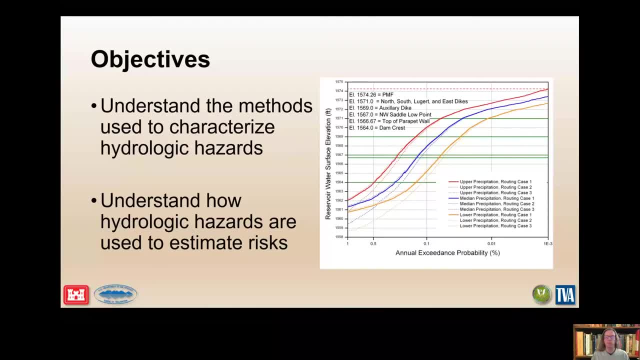 We'll focus on two objectives: hydrologic hazard methods and how they're used. The figure shows a hydrologic hazard curve, In this case a reservoir stage frequency curve for Altus Dam in western Oklahoma. Here we show reservoir water surface, maximum reservoir water surface on the y-axis and annual exceedance probability on the x-axis. 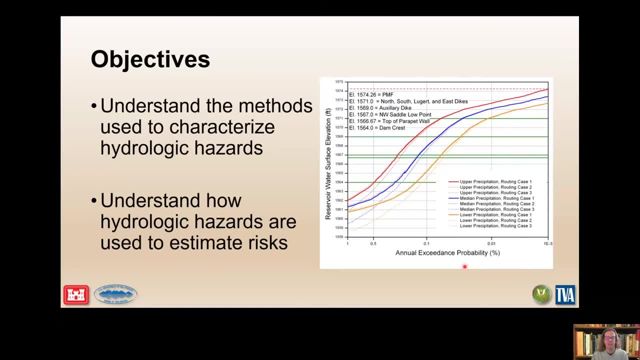 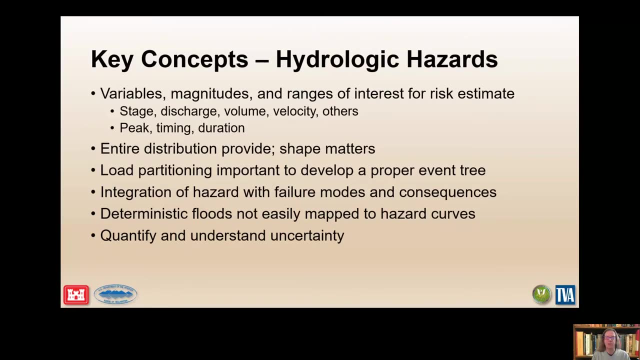 You'll see a lot of these pictures over the next several slides and we'll use these to describe how hydrologic hazards are used to estimate risks. Here are the key concepts up front. We'll discuss these along the way. Hydrologic hazards depict important variables, usually reservoir or river stage, peak discharge flow, volumes or duration. 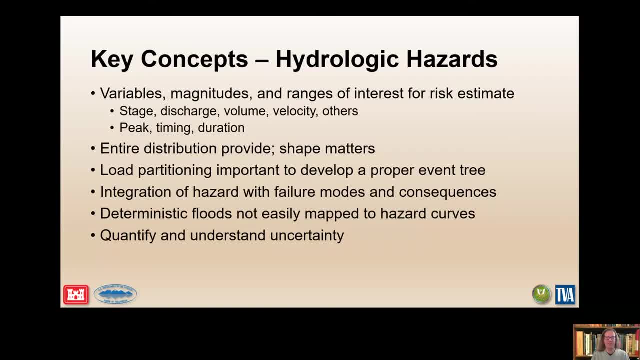 The hazard curve provides a complete distribution for static and hydrologic potential failure modes. The shape matters. They also can be used for seismic hazards. You need to target the hazard estimate to address particular failure modes and consequences. Deterministic or design floods are not used in estimating hazard curves. 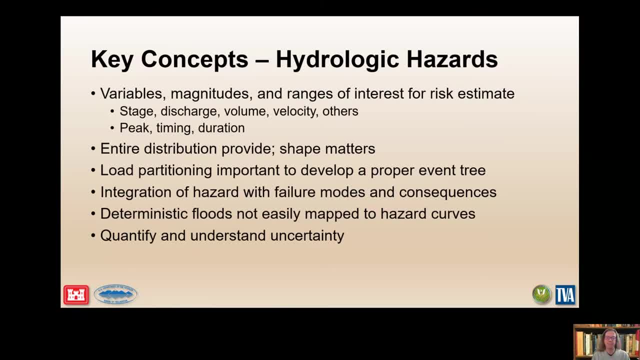 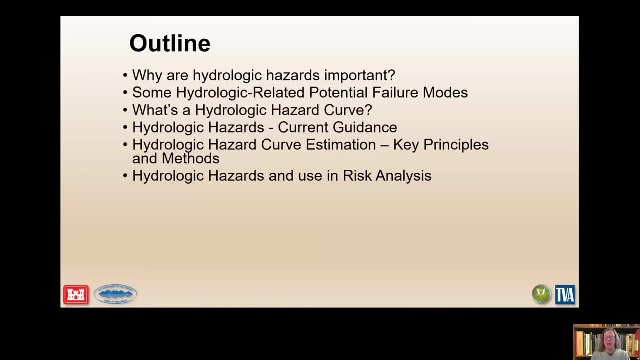 Uncertainty needs to be quantified. Here are the ideas we'll cover in this talk: What are hydrologic hazard curves and why are they important? Some potential failure modes: What is a hydrologic hazard curve? Guidance, principles and use. 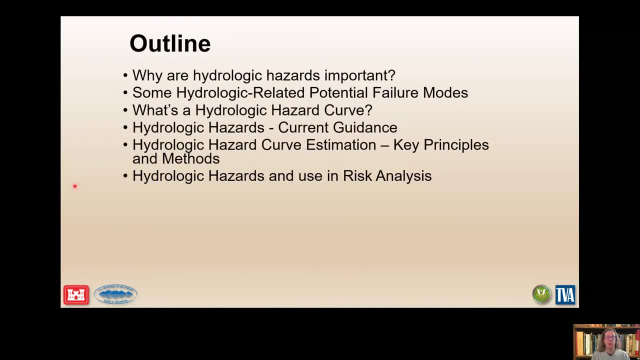 You should note Chapter B1.. Chapter B2 provides a ton of references, electronic links to publications and software and lots of details. Please be aware of it. This presentation really is just an overview. The chapter has important details for those estimating hydrologic hazards. 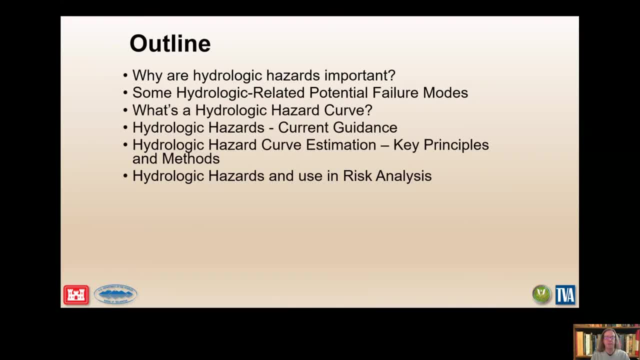 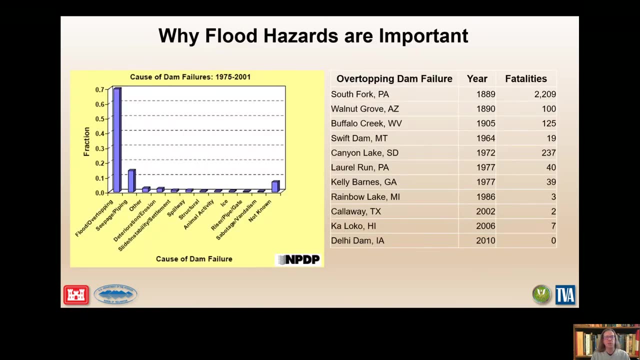 Along the way in this talk we'll show you some hyperlinks that can be directly connected to data sets, software and publications for reference for you to use in your studies. So a large fraction of dams, particularly embankments, have failed due to overtopping. 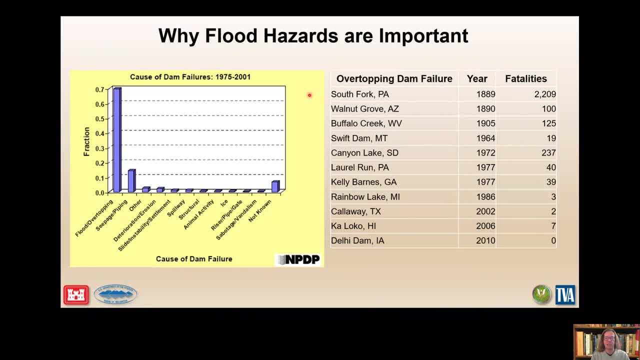 Flood hazards are the key to estimating overtopping risks. Some dams that have failed from overtopping are listed in this table. Many of you may be familiar with the Johnstown Flood. This is South Fork Dam in Pennsylvania in 1889 where over 2,000 fatalities occurred. 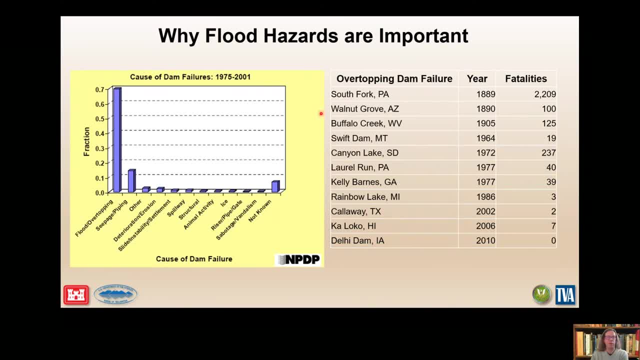 And several other famous cases: Buffalo Creek, Coal Mine Dam failure in West Virginia, A big flood in Montana in 1964 in June, Swift Dam, Laurel Run in Pennsylvania. We'll show you some pictures on that one. Kelly Barnes Dam in Georgia. 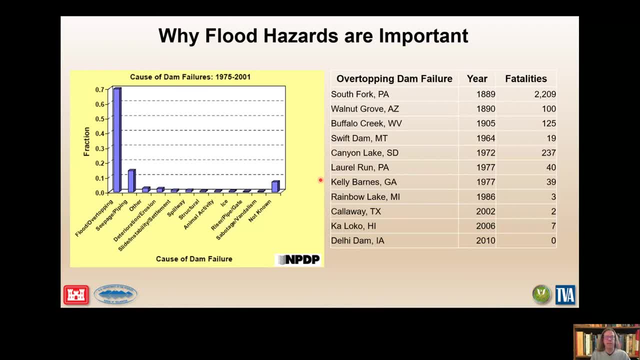 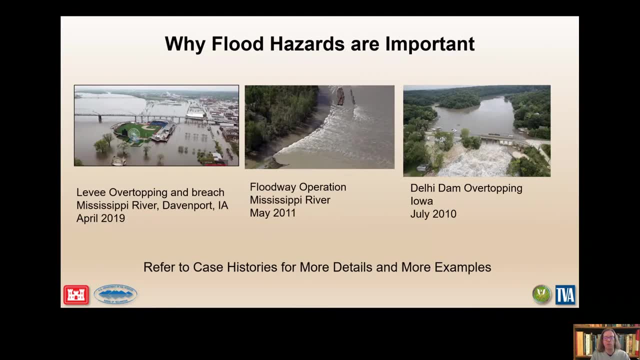 Many of these are all triggered by extreme rainfalls and have caused loss of life. Here are three examples illustrating why flood hazards are important. From left to right, we have levy overtopping and failures during the April 2019 floods. Here this is in Davenport, Iowa, along the Mississippi River. 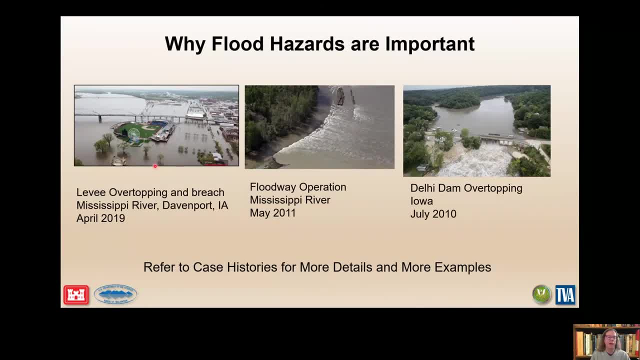 Notice the stadium in the foreground here. The river wasn't as high as it was in June 1993, but they still have challenges with protecting downtown Davenport with levees during large floods. The middle picture, Bird's Point, New Madrid levee on the Mississippi River. 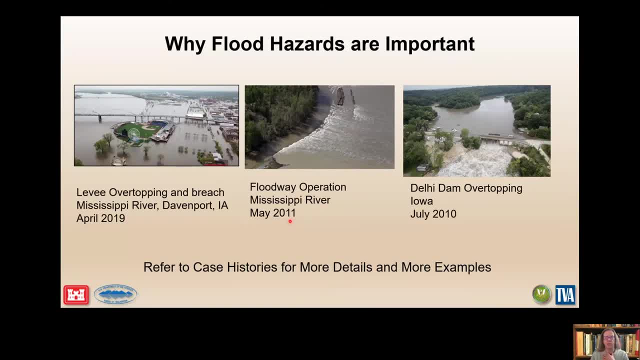 Ohio River as well, in operation. And then the third picture is Del High Dam in eastern Iowa and a dam failure that was caused by overtopping Lots of detail in our case, histories that the Bureau of Reclamation and the Army Corps of Engineers have on file, as well as FVRC. 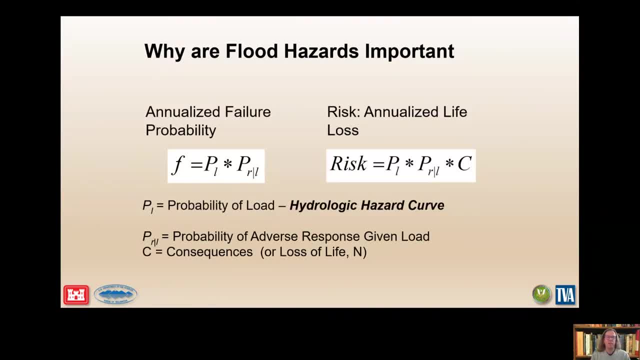 So why are flood hazards important? This talk will focus on the probability of the flood. Notice the load probability. we term it PI here or PL in these two equations. Clearly it is an equally important contribution for annual failure probability and risk. 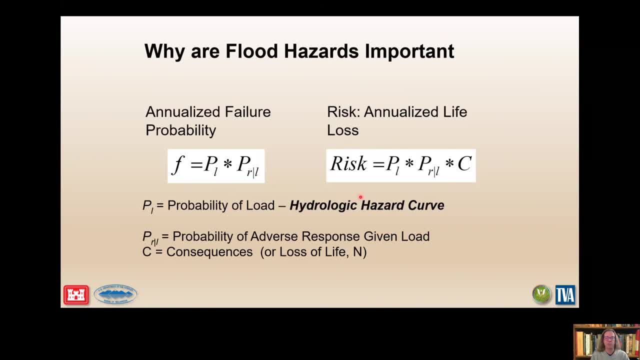 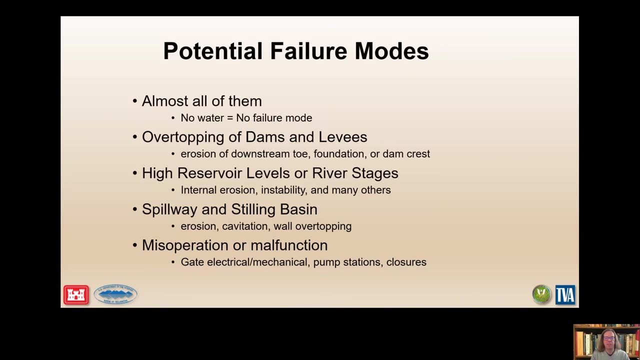 We'll focus on the hazard curves for the rest of this presentation but realize the response, probabilities and consequences are covered in other best practices lectures. Hydrologic hazard curves provide magnitude-sensitive data for flood hazards. They also provide magnitude and probability estimates to assess risk for nearly all failure modes. 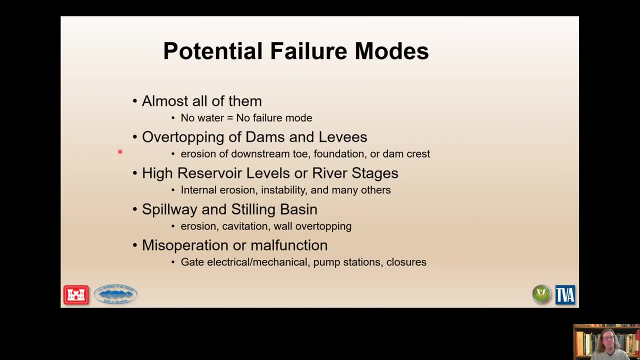 Here are some key examples: Overtopping Internal erosion, Spillway erosion leading to failure, Spillway chute wall overtopping, High reservoir levels that can compromise or cause gate issues, and others. Again, best practices presentation cover many of these potential failure modes. 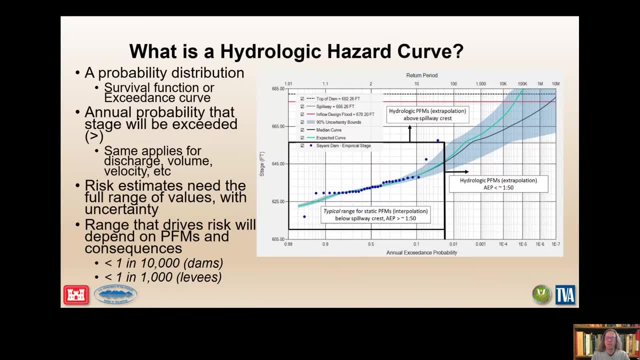 So what is a hydrologic hazard curve? It is typically a graph of reservoir elevation stage, as shown here, versus annual exceedance probability. for dams, For levees, they usually depict river stage. Hydrologic hazard curves also can show peak flows, flood volumes or stage durations versus annual exceedance probability. 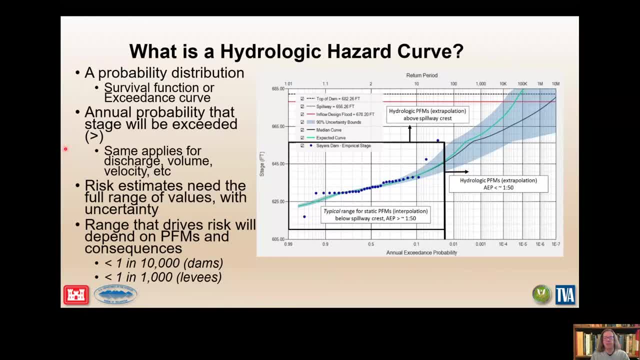 Notice the significant extrapolation beyond the annual exceedance probability. This is an extrapolation beyond the observed reservoir stages shown here in these blue dots, to the very, very small AEPs needed for dam safety, Levee safety. not so much extrapolation, but still we want to be in the 1 in 1,000 to 1 in 10,000 annual probability. 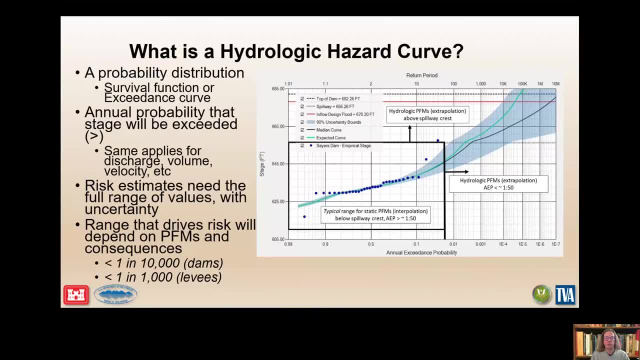 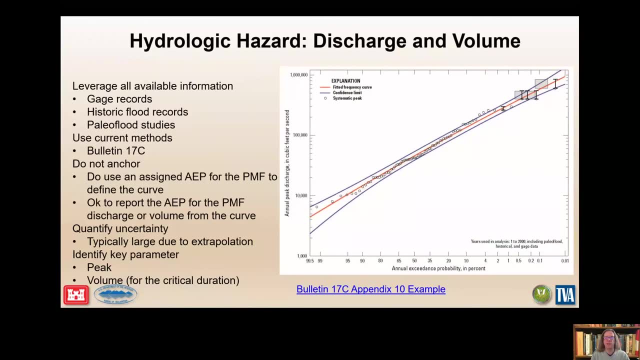 Extreme storm rainfall, historical flood data and paleo flood data with hydrologic models and statistics are used to estimate these curves. We'll cover these items in due course. Here's an example of a hydrologic hazard curve showing peak flow versus the annual exceedance probability for Folsom Dam on the American River near Sacramento, California. 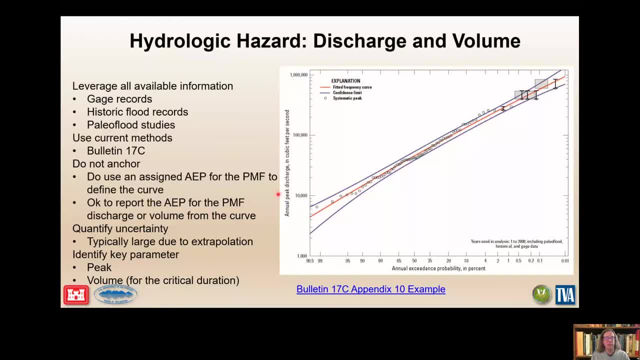 Some details are in the National Flood Frequency Guidelines report BOLTN17C. Here's a hyperlink to that appendix with the example and the document itself. This data set includes a long gauge record, A large historical flood and paleo floods shown here as flow ranges and gray boxes. 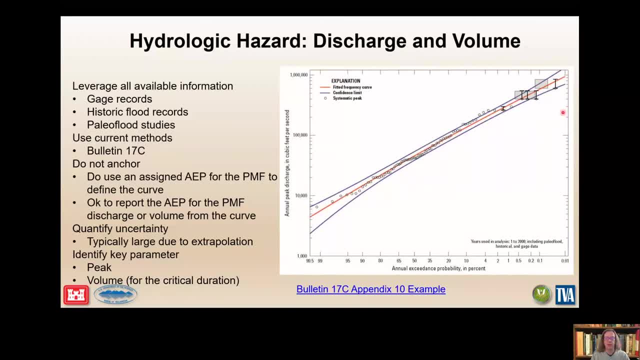 These data are critical to extend the record in time here about 2,000 years and reduce the bias and uncertainty in the extrapolations. So notice we have for bias the curve that is shown in red here, as opposed to being down here too flat or up here too high. 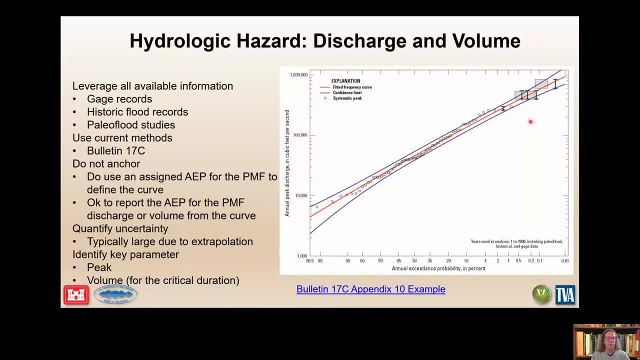 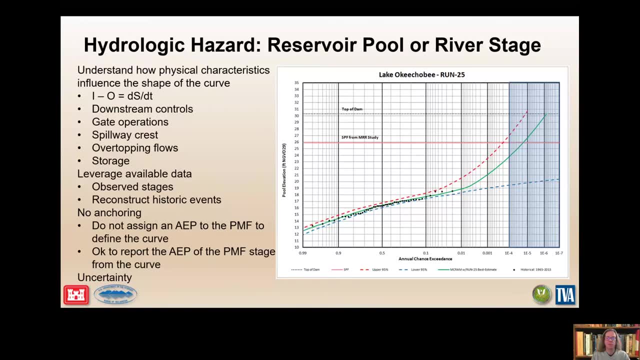 And uncertainty is essentially the width with these confidence intervals. Here's an example of a hydrologic hazard curve showing maximum reservoir stages for Lake Okeechobee in Florida. This hazard curve is based on a stochastic rainfall runoff model that uses all available data in the watershed. 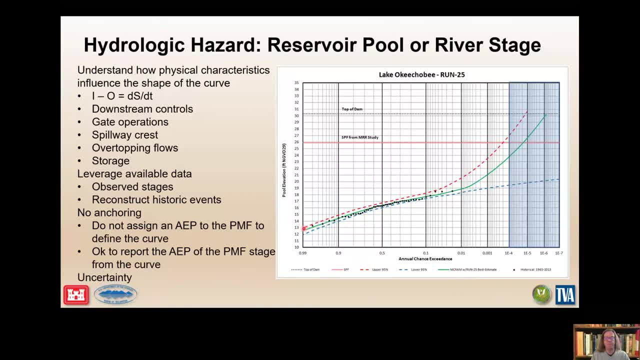 It also includes some wave runup as well in this very, very large lake in South Florida. Flows are routed through the lake, accounting for reservoir storage and outflow characteristics, which gives the curve this shape. This is the important features that you want to include in hazard curves, especially for dams: to know how downstream controls and storage and gate operations affect and can be portrayed in the hazard curve. 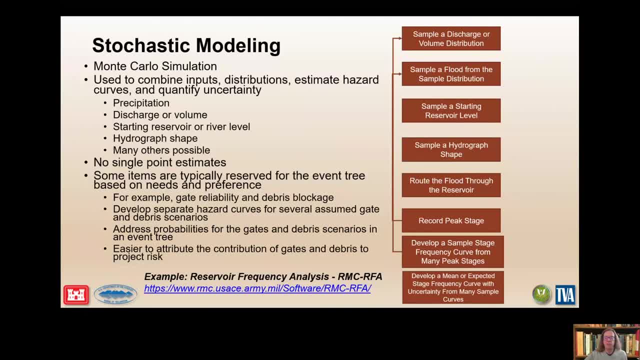 Monte Carlo simulation is used to combine inputs, For example reservoir stages, hydrographs, storages, the distributions such as flood volume and estimate hazard curves with uncertainty. A flow-based Monte Carlo sampling scheme is illustrated in the flow chart here on the right. 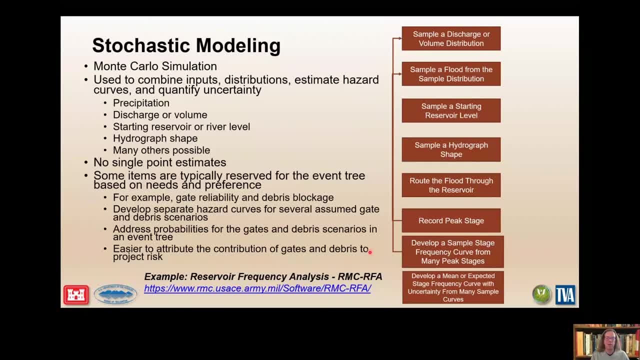 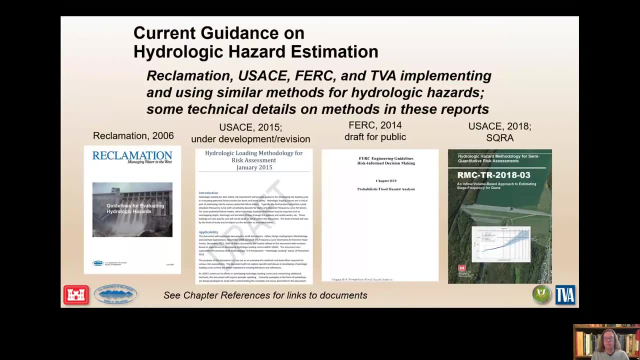 These are the main ingredients in the RMC-RFA software, Reservoir Frequency Analysis, used to estimate reservoir stage frequency hazard curves. Again, a link is shown here directly to the software with the user's manual and some examples. Hydrologic hazard methods and applications for dam safety started at the Bureau of Reclamation principally in the late 1990s. 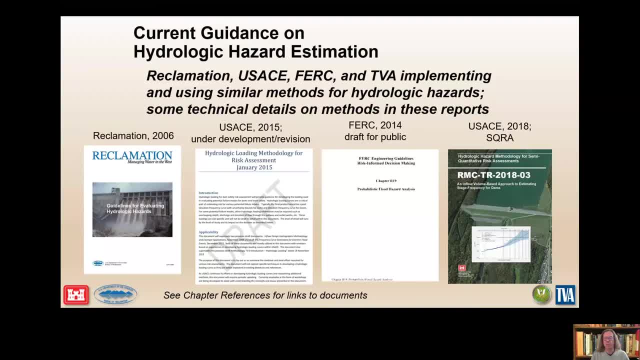 Although risk has been used for many, many years, since, essentially, the inception of American Society of Civil Engineers in the 1870s. Over the past 20 years, in particular, the four major federal agencies in dam safety- the Bureau of Reclamation, Army Corps of Engineers, Federal Energy Regulatory Commission and Tennessee Valley Authority- as well as the Nuclear Regulatory Commission, have performed research and developed similar methods on hydrographic hazard. 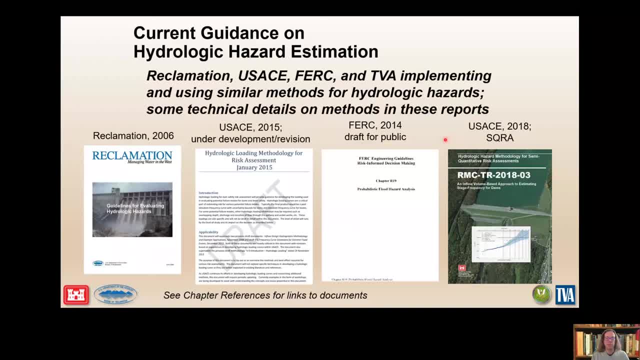 Similar methods on hydrologic hazards, also known as probabilistic flood hazards. These reports contain key technical details. You can get the references for these in your chapter. You can also find lots of good references on the web, as the Nuclear Regulatory Commission has been hosting probabilistic flood hazard workshops since 2013 on this very topic. 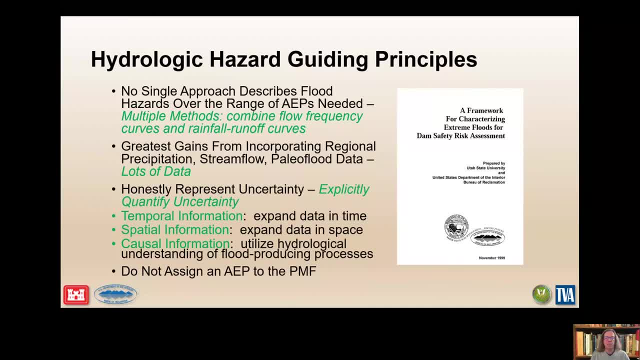 This 1999 report from the Bureau of Reclamation and Utah State University presents some guiding principles for how to perform these research and development strategies. Here are some of the results we use today: Combining flow and rainfall runoff hazard curves, adding lots of data. 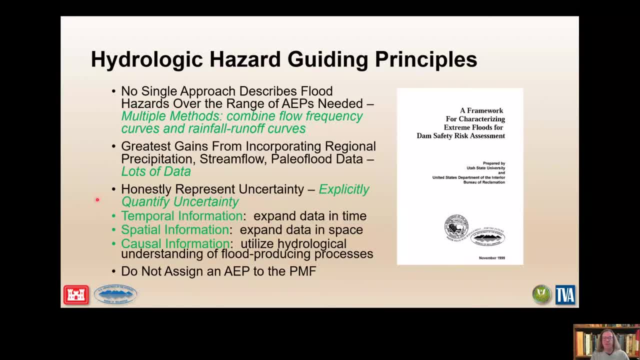 quantify uncertainty, expand data and time with, say, historical and paleolithic information. Do spatial information include that such as regional precipitation frequency? We need to be deliberate to include each concept and include more information on hydrological processes and hydrological reasoning which falls under causal information. 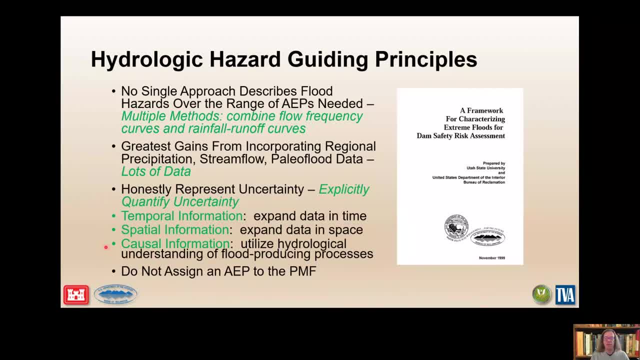 Are extreme floods and storm data representative of the extreme processes we're trying to predict? Combining data evidence from each piece is the key to do this. You can look at the references in the chapter, such as Mersham-Bloschel and a couple of papers. 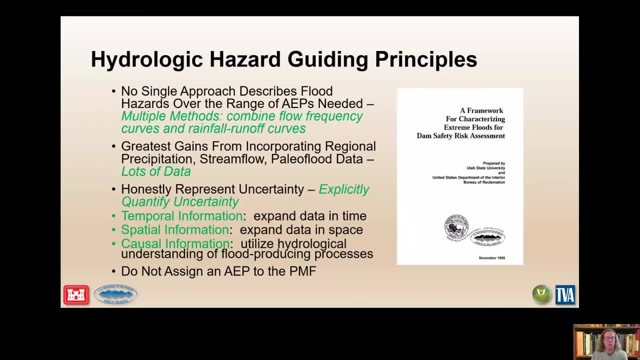 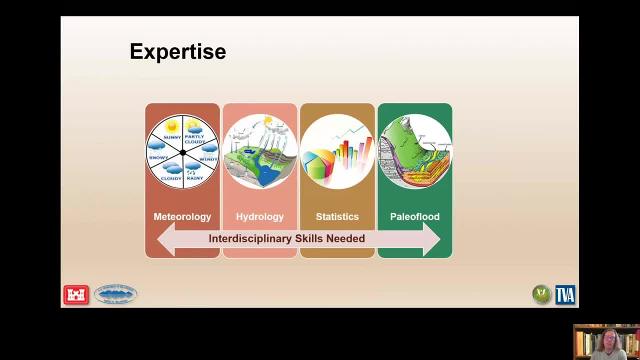 in Water Resources Research, as well as the National Research Council publications, which we've used extensively over the years, And it takes a team with specific specialties, training and expertise to collect data and estimate hydrologic hazard curves, Meteorology, Storm, rainfall data analyses, temporal and spatial. 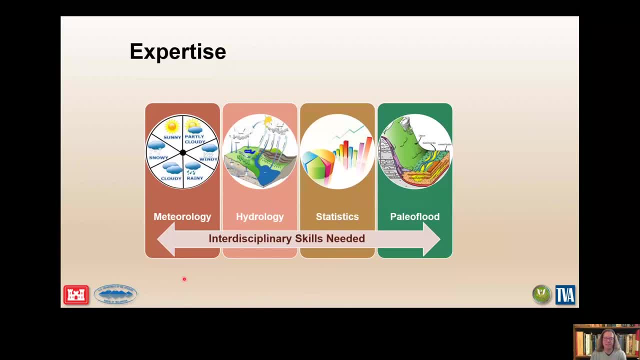 patterns of rainfall, hydro meteorology statistics, extreme precipitation- they're all key things. under meteorology There's some overlap with hydrology, but hydrology, hydraulic engineering, knowing rainfall, runoff processes and snowmobility is key. snowmelt and how the rainfall transforms to runoff and the timing of that in your watershed. 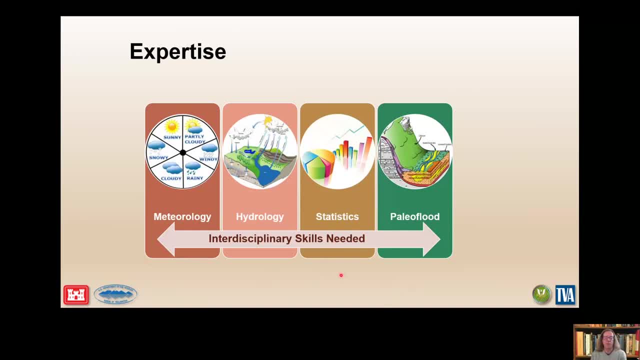 is critically important Statistics. We do lots of statistics with flood frequency, flood statistics, stochastic models and precipitation frequency analysis. Paleofloods include geology, fluvial geomorphology, hydraulic engineering to look at past records of very, very large floods, which are also critically important. 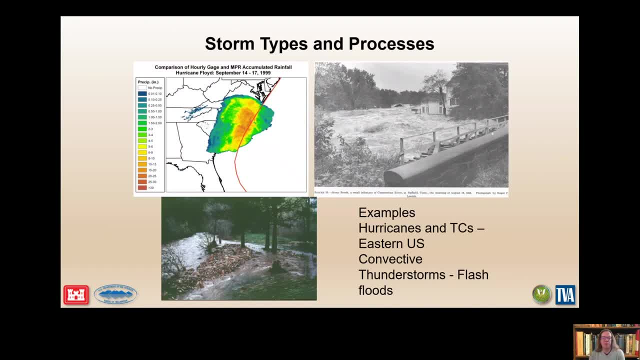 Here's an example of interdisciplinary expertise in using knowledge of storm types and flood processes. So hurricanes and tropical cyclones are a critical dominant factor along the east coast, important drivers of floods. With Hurricane Floyd shown here, this is a picture of rainfall. 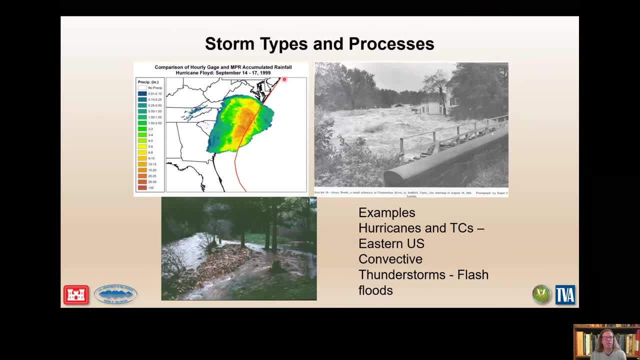 depths in inches, with the storm track going up the east coast, focusing on North and South Carolina. from multi-sensor precipitation reanalysis data Here on the left-hand side of the slide, we have a picture of a storm track going up the east coast. 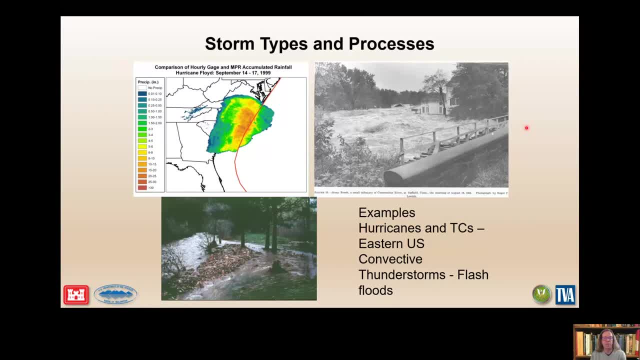 Here on the right is flow depths and this river, actually Stony Brook, next to this 1850s farmhouse. next to the August 1955 flood in Connecticut, Seven US Army Corps of Engineers dams were built after the 55 floods in Connecticut in the Naugatuck River Basin. nearby Flash floods are an important 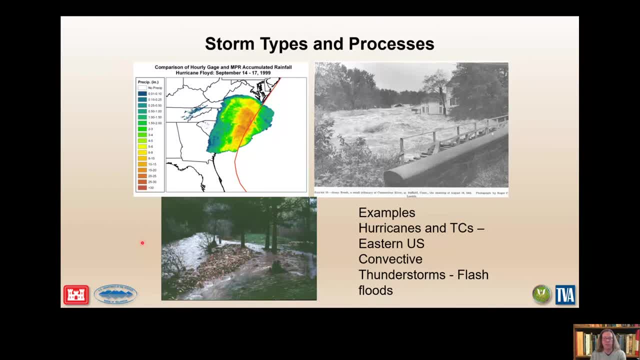 process in many watersheds here in the western US, shown by this boulder bar and left-hand creek near Lyons, Colorado, looking upstream here. So it's important to integrate rainfall, flood runoff processes and what's happening in the stream channel itself with fluid geomorphology to describe. 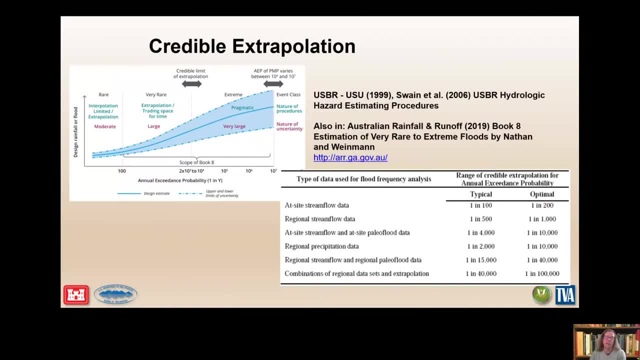 these flood processes and hazard curves? What about extrapolation? It is critical to collect multiple data sets and lines of evidence for credible extrapolation of a hazard curve. In general, our instrument records are fairly short, on the order of about a quarter of a second. 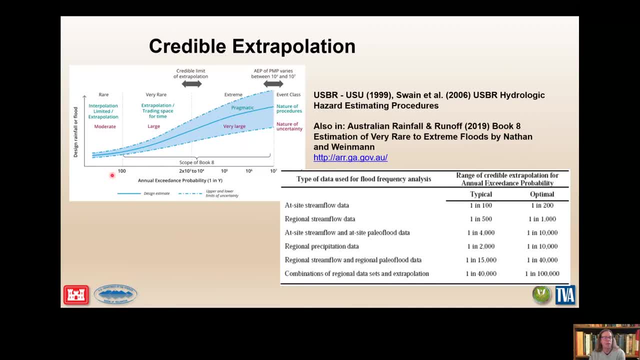 So we use regional precipitation, regional streamflow and paleoflow data to do this extrapolation. Extrapolation of a reservoir stage record or a streamflow gauge is simply insufficient at your site of interest. A couple of important links here are to the Bureau's Hydrologic Hazard Curve Estimating Procedures Report. 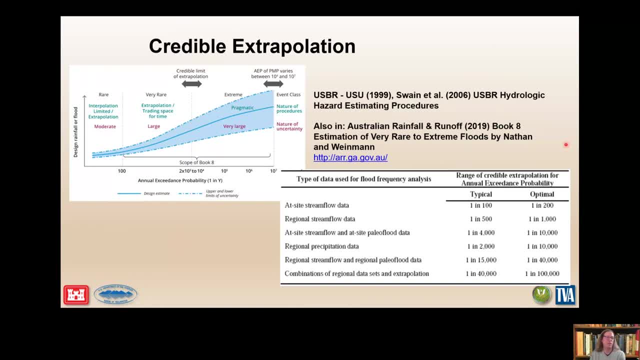 And also some details. This figure on the left is from Australian Rainfarm Roth. We've closely collaborated with folks there over the years And this is a report on the hydrologic hazard curve. This is a report on the Australian rainfall rough. We've closely collaborated with folks there over the years. 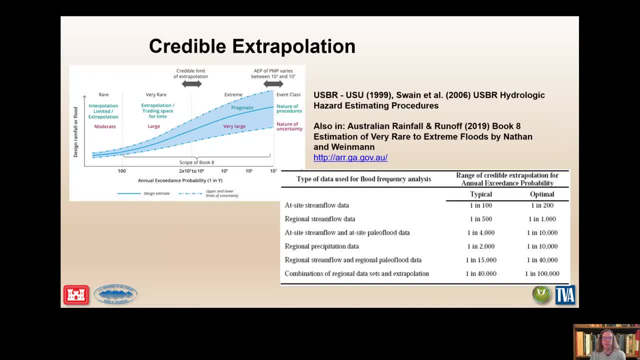 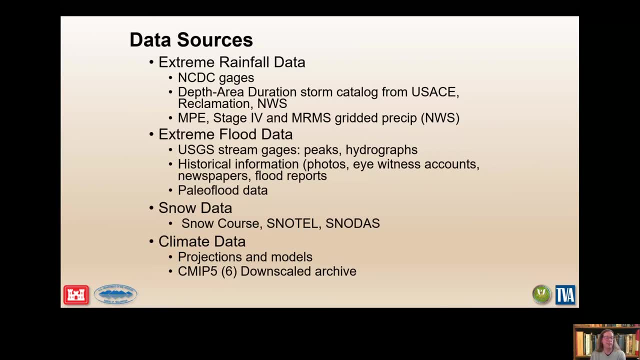 years and used and shared some knowledge and information back and forth between the agencies. data sources, data, data data. the key data sources used to estimate hazard curves are shown here. let's start with rainfall. most are from the national climatic data center, or ncei. now 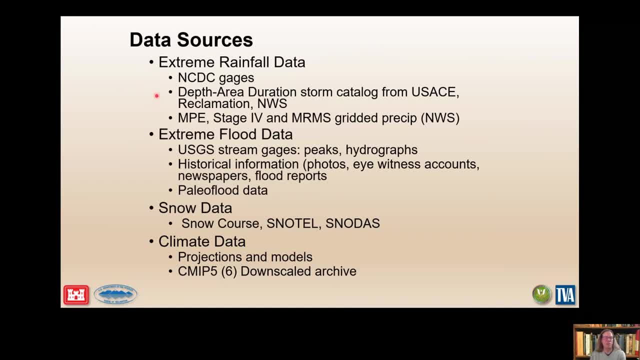 depth area duration, storm catalog from the army corps of engineers, bureau of reclamation and national weather service and critically find space and time radar and rainfall merge. products from the weather service could be multi-sensor precipitation estimates, stage 4 radar or mrms extreme flood data- critically important as well- from the usgs with historical information. 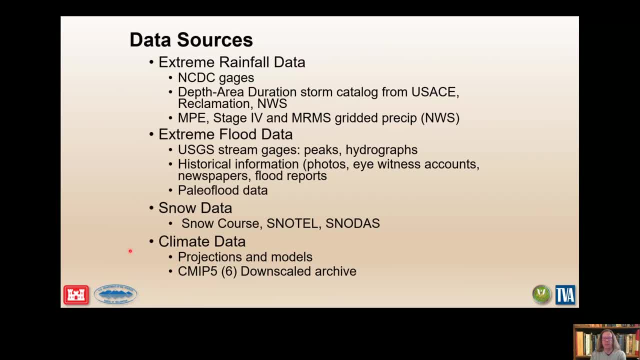 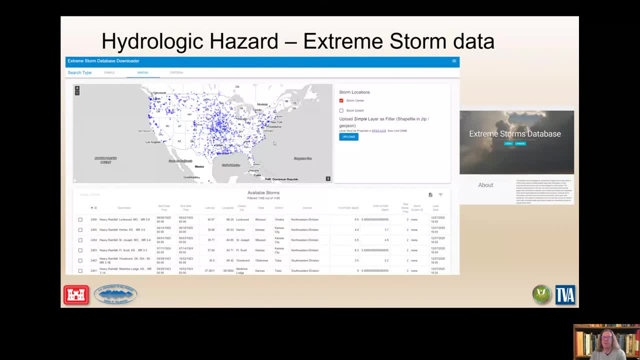 and some paleo data. snow data and climate data are also critically needed as well. here's an example of storm rainfall data from the army corps of engineers extreme storm database. there's over 1900, 1190 events- excuse me- in the database. most have been used as the basis for. 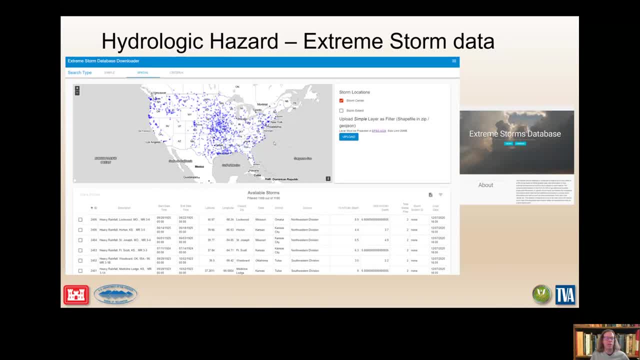 problem maximum precipitation and design rainfall at usace dams. so these storms in this database are the critical ones that were used to design uh nearly all of particular core facilities, as well as many others like the bureau of reclamation. access to the database is 밑ed to internal use. we anticipate public access within the next year. 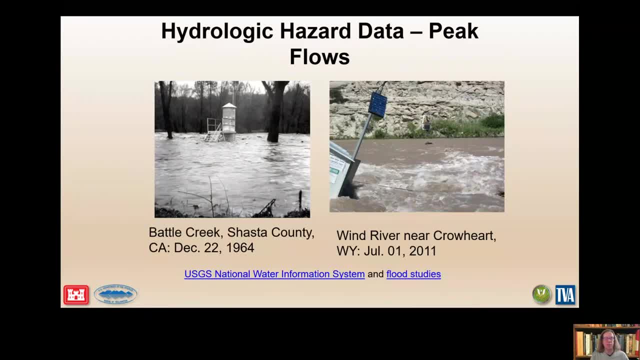 streamflow data from the usgs is critical for flood hazards. they do a fantastic job at doing streamflow measurements, rating curves and archiving data. both of these pictures illustrate floods above the rating curve for the gauge, so it's critically important to understand data collection methods, limitations, and quantify uncertainty and discharge estimates. 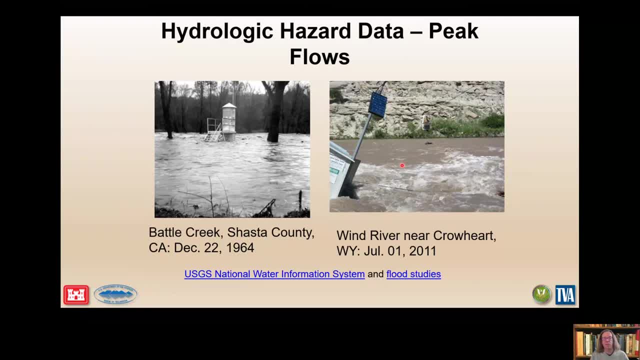 So here on the right and on the Wind River, we see a USGS hydrographer in the cable car- Notice the cable across the Wind River here- making a current meter measurement with the current meter shown here. USGS flood reports are also an invaluable resource and links are here for your handy. 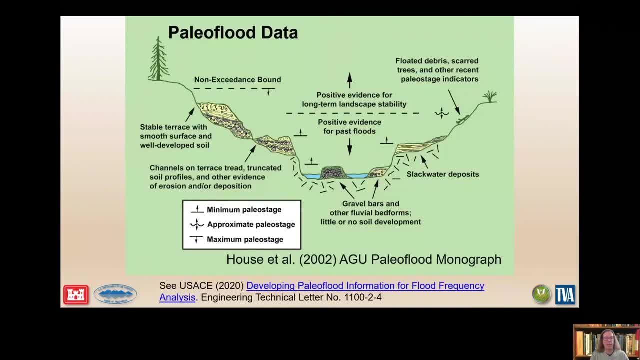 reference. Paleo flood data provide direct physical evidence of extreme floods larger than those in the systematic or historical record. Those are most valuable. The data also provide potential limits to flood magnitudes. over time, Say over the past two to three thousand years, we've had long history of stable terraces and development. Paleo data increase the effective. 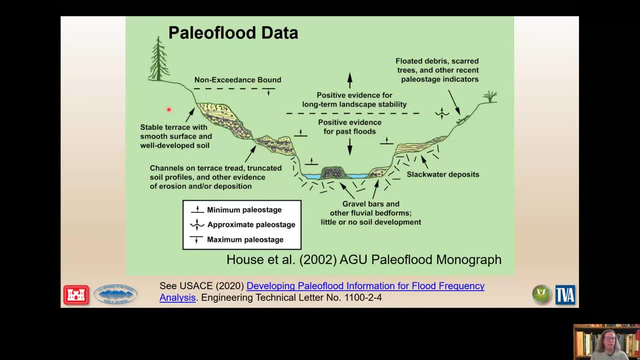 record length of floods and improve flood efficiency. The data also provide a lot of hydrologic hazard uncertainty estimates. The Corps of Engineers, through headquarters, recently released an engineering technical letter. The reference is down here, so I encourage you to become familiar with that and use the paleo data for flood risk management and dam and levee safety. 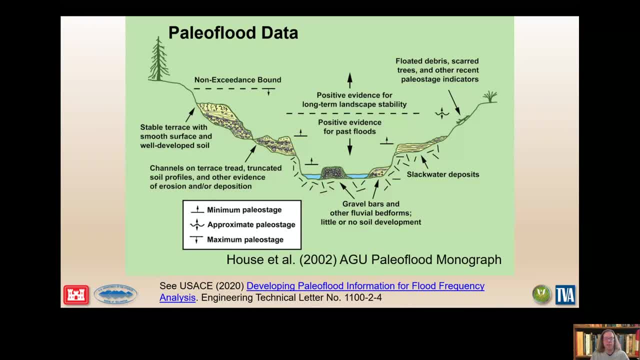 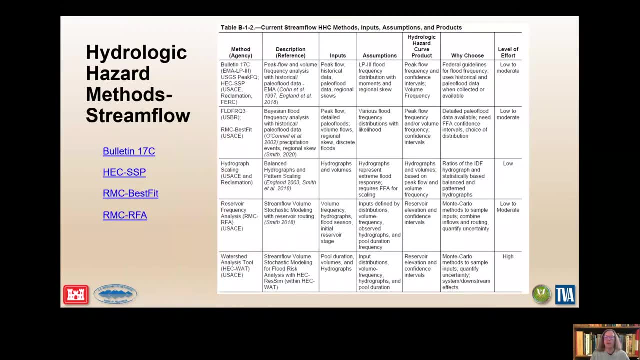 practices in the Corps of Engineers. Reclamation has had a long history of using paleo data for the past about 25 years. Hydrologic hazard methods are classified based on their major input: Stream flow or rainfall. Here is a current list of stream flow based methods. Hyperlinks listed. 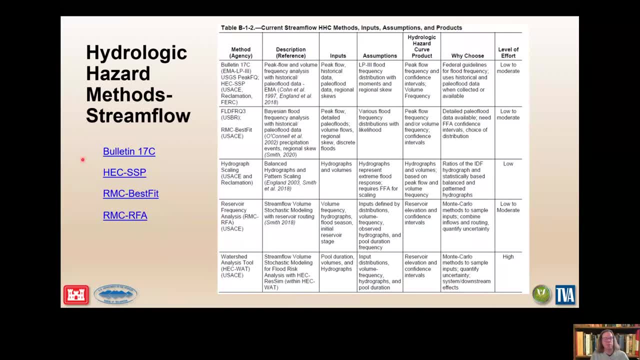 on the left provide you reports, software and manuals. BOLTON 17C is a federal flood frequency guideline and used in HEC-SSP. The Bayesian estimation and fitting software, RMC-BESFID for flood frequency includes historical paleo flood data, precipitation events and regional skew. 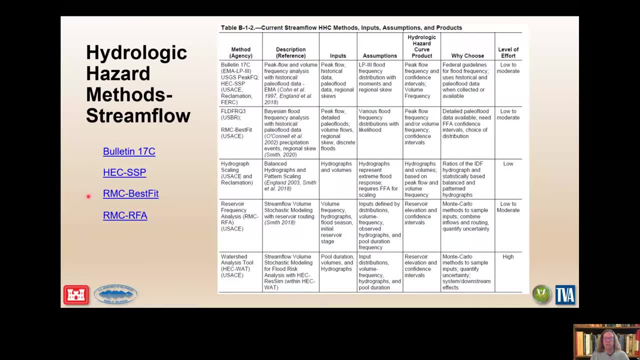 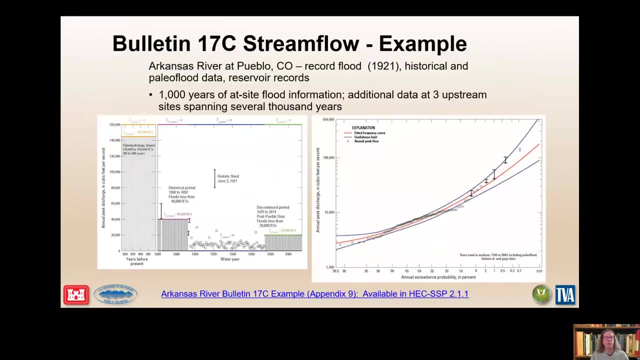 in combination to estimate a flood distribution. The Reservoir Frequency Analysis software, RMC-RFA, is used to estimate reservoir stage frequency curves. While these are all flow-based methods, we then combine them with precipitation or rainfall runoff based methods. Here is an example of a peak flow frequency. 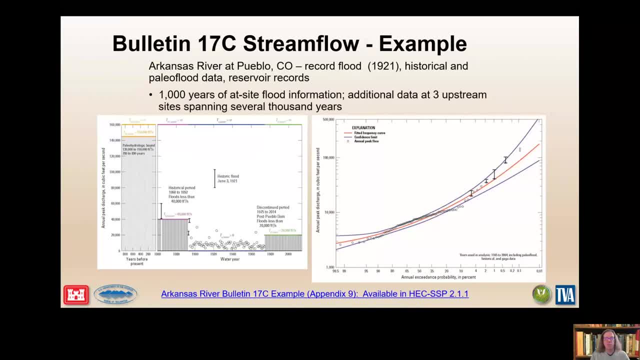 curve with historical and paleo flood data. The 1921 devastating flood resulted in over 200 deaths near Pueblo, Colorado. Pueblo Dam by the Bureau of Reclamation was constructed in 1975, in collaboration with the Corps, with a flood control pool to contain this. 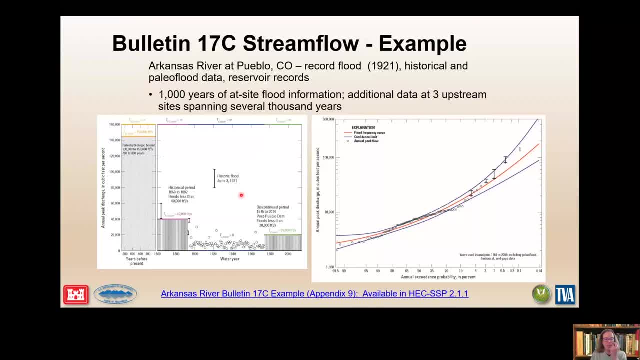 very, very large flood. It was the largest flood at the time in US history and there are many reports written after it and how to do regionalization on flood and flood frequency curves in the mid 1920s, principally led by Alan Haison. Notice: historical and paleo flood data. 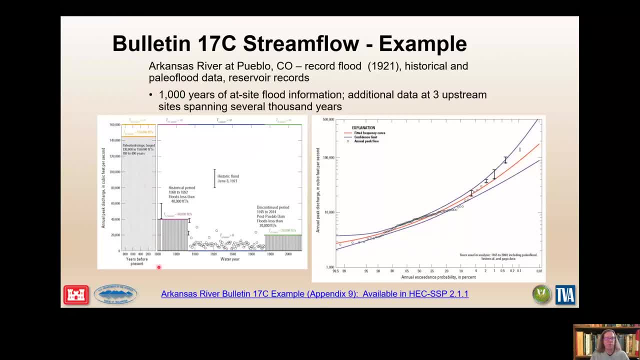 historical data shown here dramatically increases the record length back to 1859. Then, additionally, about thousand years before present, with a non-exceedance bound. These data help to provide context and reduce uncertainty in the hazard curve for very, very small probabilities. 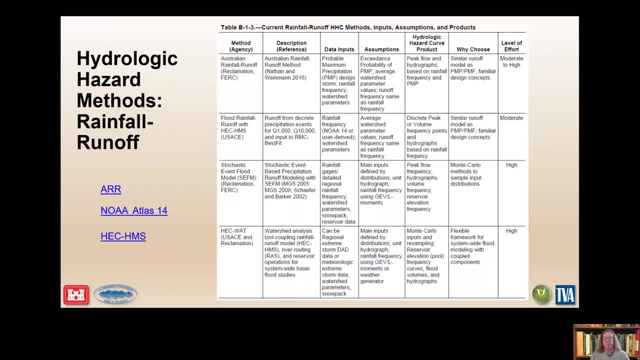 Here is a current list of rainfall runoff based methods. Details again are in your report chapter with all the references therein. Hyperlinks in the left provide your reports. precipitation frequency estimates, software and manuals. Flood runoff hydrographs, peaks and volumes are estimated from HEC-HMS with precipitation frequency estimates from NOAA. 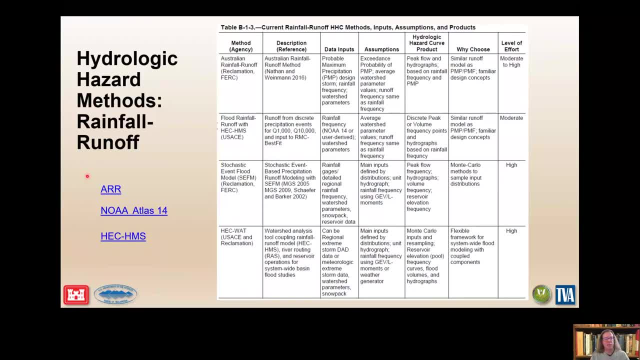 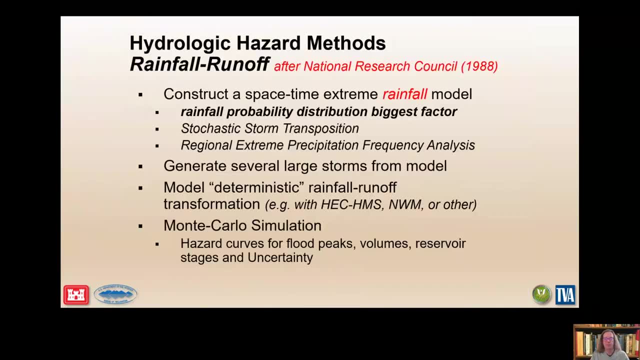 Atlas 14 or user-derived estimates. That's the key approach we're using now. Some parallel concepts are in the Australian Rainfall and Runoff Guide. Mining color simulation we use with rainfall runoff models to estimate flood peaks and volumes. This is an example of what we can do in the Australian Rainfall and Runoff Guide. 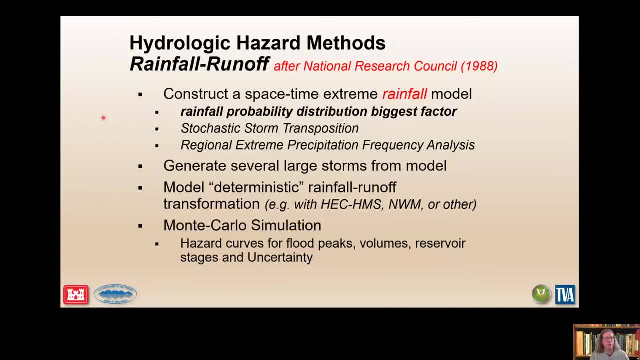 Mining color simulation we use with rainfall runoff models to estimate flood peaks and volumes. This is an example of what we can do in the Australian Rainfall and Runoff Guide. The main input is a rainfall distribution, so the probabilities really come from rainfall with spatial and temporal patterns, Several extreme storms are generated, then floods are. 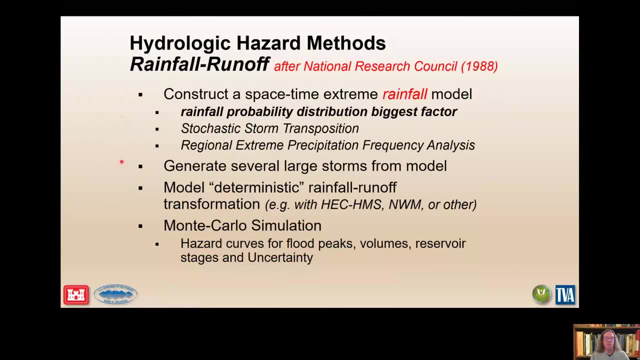 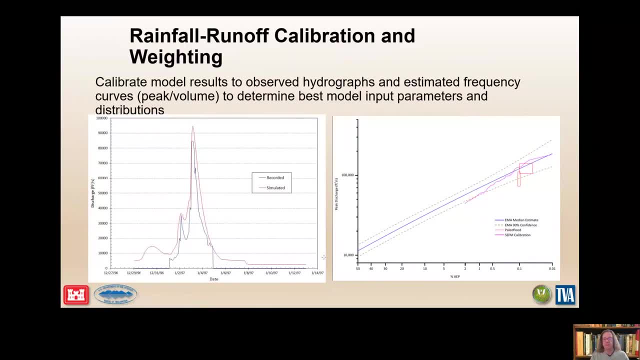 estimated for each storm event. The rainfall runoff captures the physics of floods, with the transformation of rainfall to runoff and routing of floods through the watershed. A key requirement is to calibrate and validate the rainfall runoff model with the largest floods, Mining color simulation we use with rainfall runoff models to estimate flood peaks and volumes. 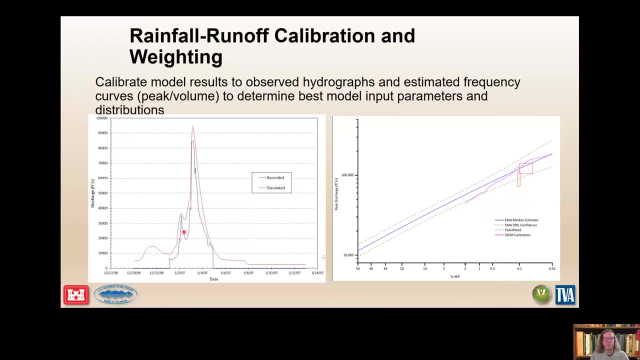 To ensure the model actually represents the flood timing, peak, volume and shape. Here's an example, from the 1600 square mile watershed at Friant Dam in California, Calibration, to the large 1997 flood shown on the left, with flood magnitudes approaching. 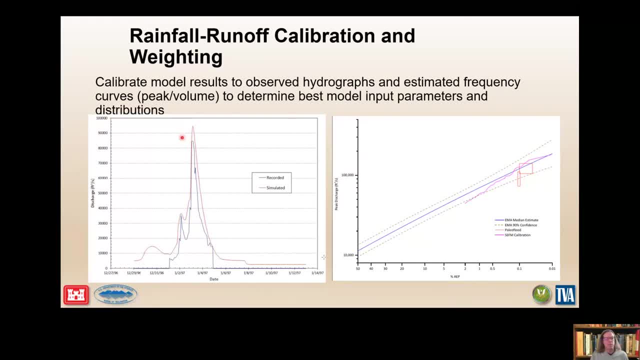 100,000 CFS. Notice that the hydrograph that's simulated from the model shown in red fairly accurately matches the timing of the flood timing Mining color simulation we use with rainfall runoff of the observed hydrograph shown in blue and the overall shape. 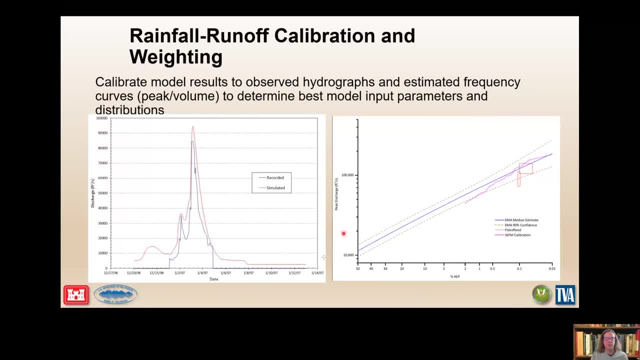 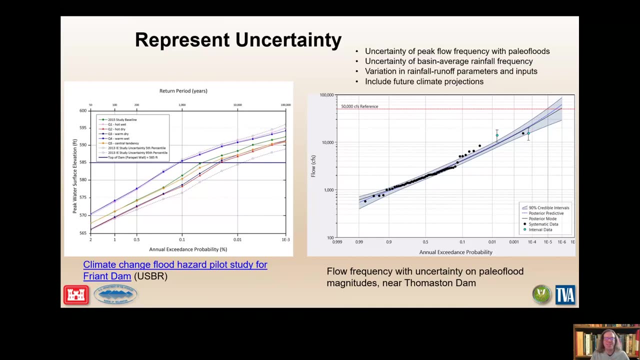 Secondary calibration can be done with a peak flow frequency curve for this case study, with historical and particularly paleo flood data shown in these red boxes here It is crucial to represent uncertainty in hydrologic hazard estimates, Uncertainty in data, flood magnitudes, precipitation in space, runoff model. 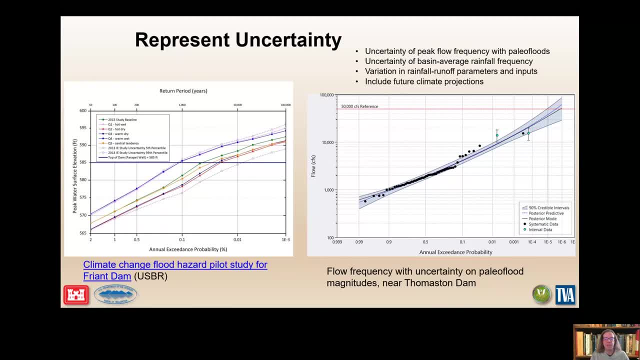 parameters, future climate and other aspects can be quantified. So here on the left we have uncertainty in reservoir stage from precipitation. There's various precipitation frequency estimates which result in these peak water surface elevations for Friant Dam, again in the Central Valley in California. Historical and paleo flood data. 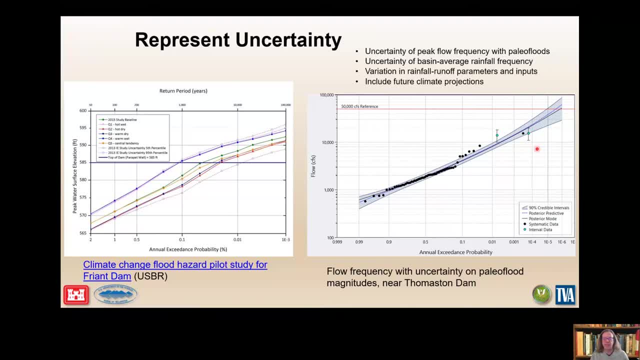 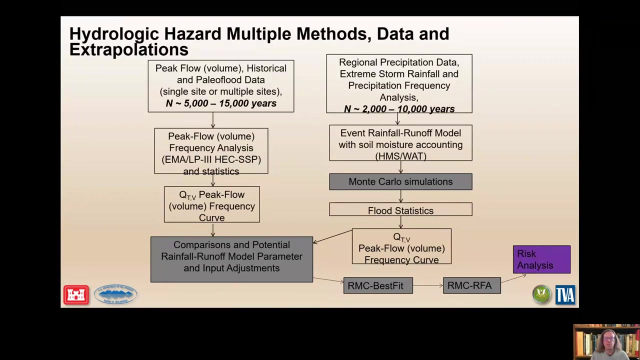 help place this August 1955 flood here on the Sheep Hog River in West Central Connecticut in proper time context and reduce help reduce uncertainties that may be applied to nearby Thomasson Dam. Here is the recommended workflow for estimating hydrologic hazards. This shows streamflow base estimates on the left: 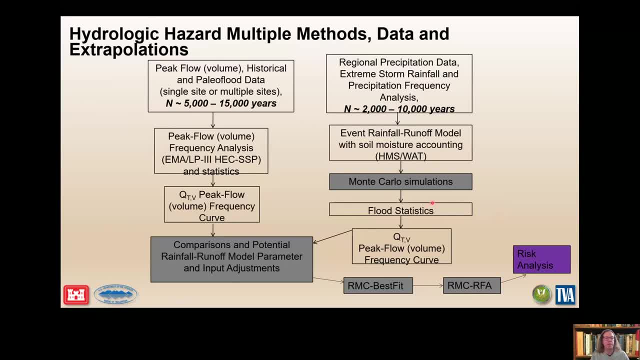 and rainfall runoff estimates on the right. Streamflow data again includes historical and paleo flood data. Rainflow runoff includes regional precipitation frequency and extreme storm rainfall. These two estimates are then combined with RMC best fit and a hydrologic hazard curve for reservoir stage is estimated with RMC-RFA Risk analysis inputs for specific. 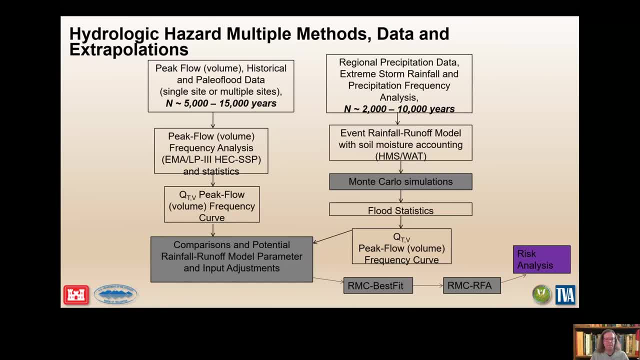 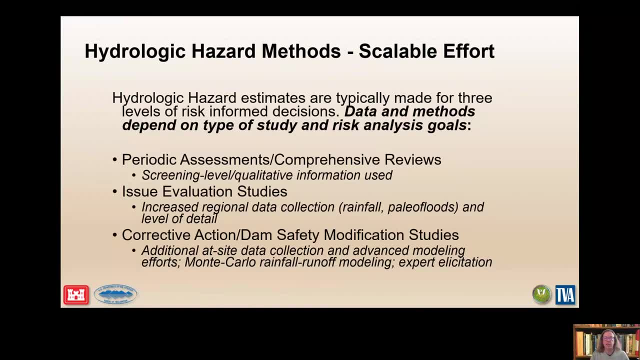 failure modes can then be obtained from RMC-RFA. It is important to realize that hydrologic hazards, hydrologic hazard data, the data collection and methods used are scalable for the risk analysis and decision being made. There are three main levels of study, as shown: Data and methods. 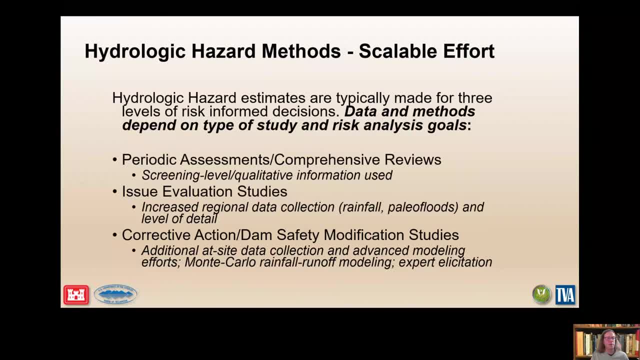 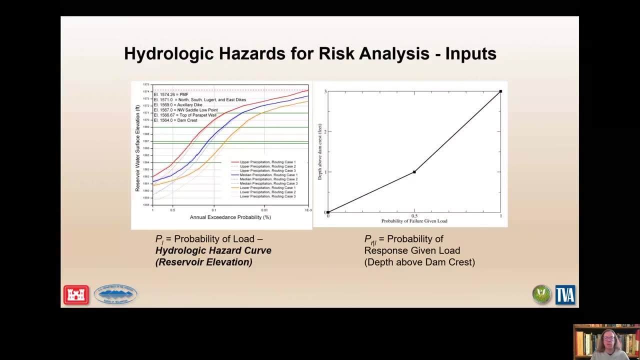 depend on the type of study and risk analysis goals. For example, issue evaluations, we spend a bit more time increasing regional data collection could be rainfall and or paleo floods and level of detail for quantitative risk assessments. Two main inputs to quantitative risk analysis: reservoir stage frequency curve shown here on the 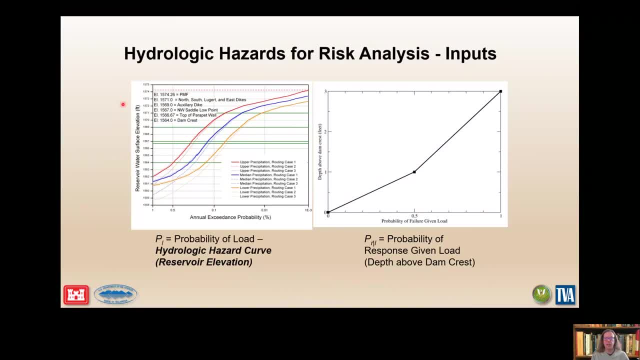 left and a fragility curve for, say, an overtopping potential failure mode. The hazard curve on the left provides the depths and the probabilities over the areas of interest. This could be the dam crest, saddle dikes or parapet wall. On the right we show an example: failure distribution for.